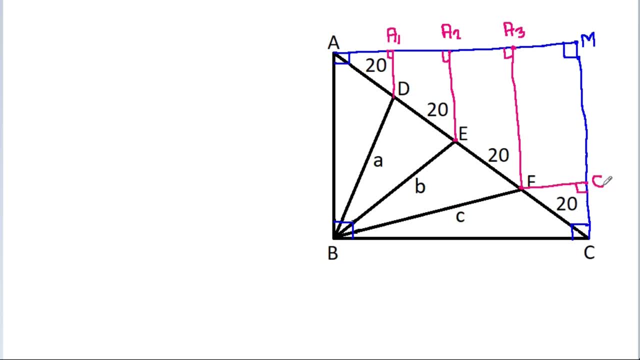 on C on CM, suppose this point is C1.. From E on CM, suppose this point is C2. And from D on CM, suppose this point is C3. Then these angles, they will be equal. suppose theta. 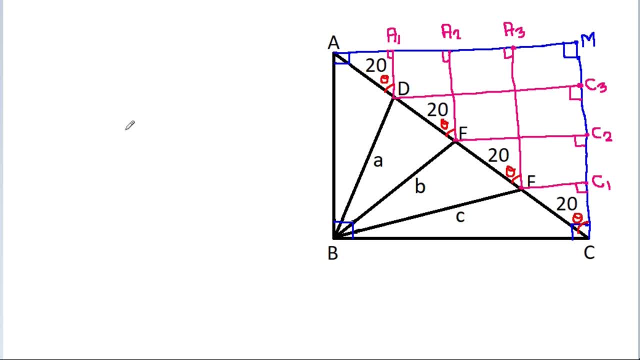 and in any triangle, if this angle is 90 degree, this angle is theta and this length is 20, then this length it will be 20 sine theta, And this length it will be 20, cos theta, And here suppose A is x. 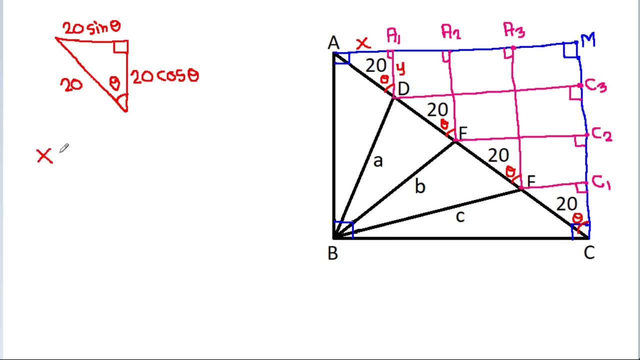 and is y, Then x will be equal to 20 sine theta And y will be equal to 20 cos theta. And again, these angles, they will be 90 degree. So this angle will be 90 degrees, 90 degree. so it will be x, it will be y, it will be x, it will be y, and it will be x, it will be y. 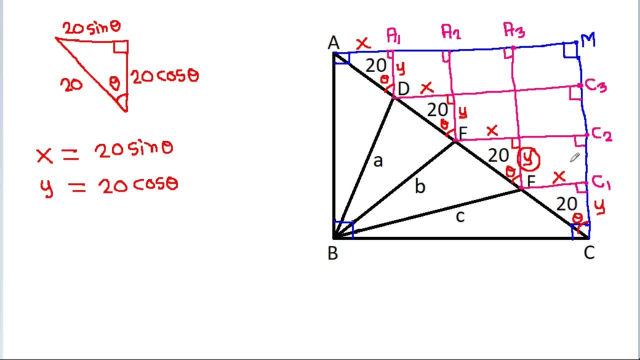 and again, this length is y, so c1, c2, it will be y, c2, c3, it will be y and c3, m it will be y, and a1, a2 it will be x, a2, a3, it will be x and a3, m it will be x. 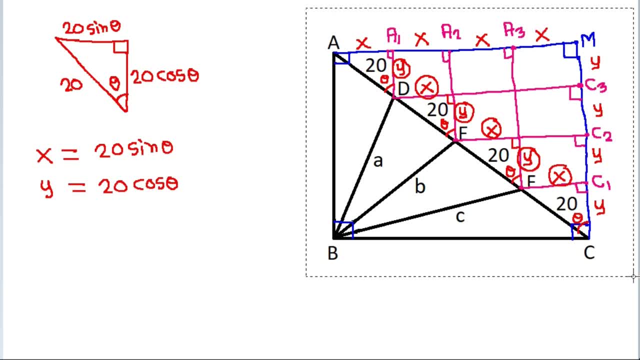 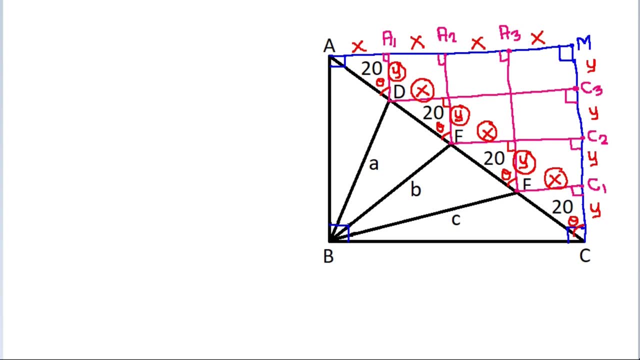 and now if we draw a perpendicular from d on bc, suppose this point is b1, then bb1 it will be equal to a1, that will be x, and db1 it will be equal to c3, c, that will be 3y. so inter angle bd. 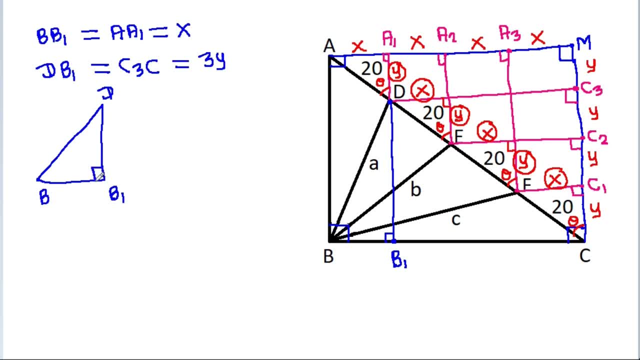 b1, this angle is 90 degree, bb1 is x and db1 is 3y and bd is a, so a square: it will be equal to x. a square minus 3y, a square by pythagoras theorem. and also if we draw a обще았어 picture from f on: 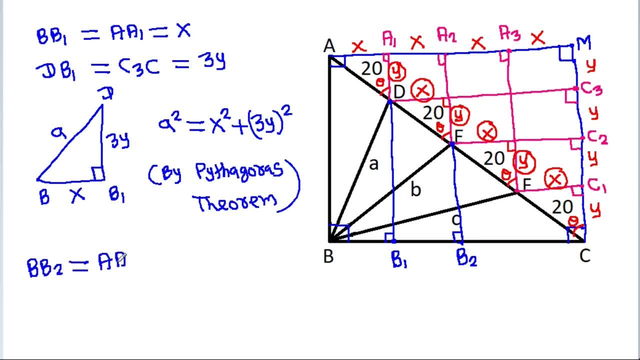 B2 it will be equal to a, a2- that will be 2x on b, c and if b2, it will be equal to a2 and the sum of the is everyone will be 2a2. then f will be equal to a2 and the sum of the wages of A2, that will be two x and sub 2 and� f, b2- it will be equal to c to c, that will be 3a1. now, this point is a contribution point. 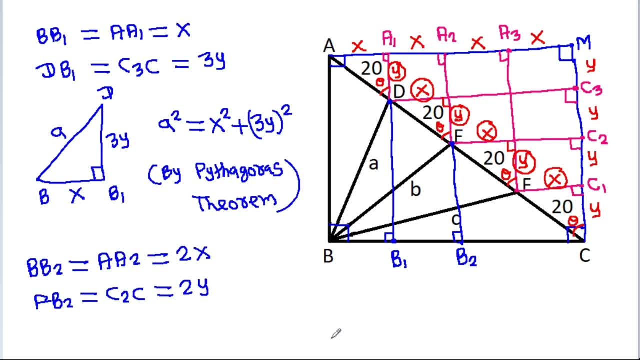 y. so inter angle b, f, b2, bf is b. this angle is 90 degree. b, b2 is 2x and f, b2 is 2y. so b square it will be equal to 2x square plus 2y square. and again in the same way if we draw a perpendicular. 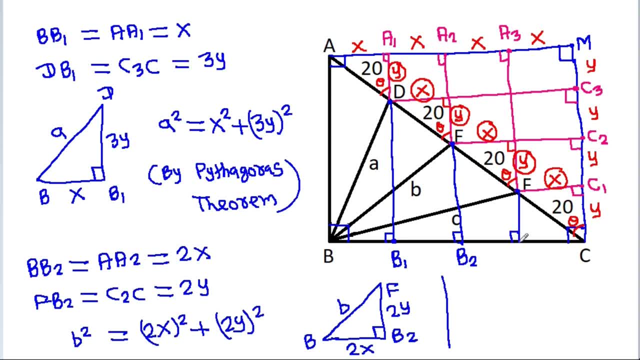 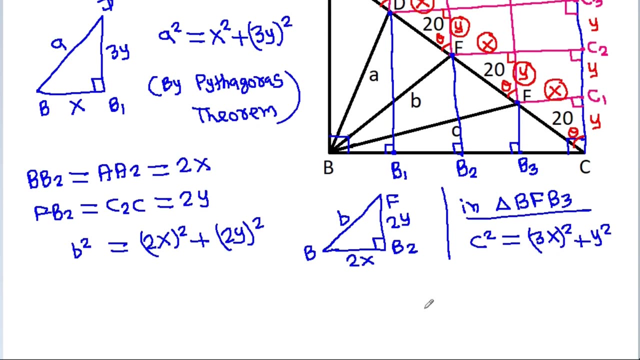 from f on bc. suppose this point is b3, then inter angle bf, b3, c square, it will be equal to 3x square plus y square. so a square plus b square plus c square it will be equal to x square plus 3y square plus 2x square plus 2y square. and again in the same way. if we draw a perpendicular from f on bc, suppose this point is b square, it will be equal to 2x square plus 3y square plus 3y square plus 2y square. and again in the same way if we draw a perpendicular from f on bc: suppose this point is b square plus. 3y square plus 2y square plus 2y square. and again in the same way, if we draw a perpendicular from f on bc, suppose this point is b square plus 3y square, plus 2y square plus 3y square. and again in the same way, if we draw a perpendicular from f on bc, suppose this point is b square.